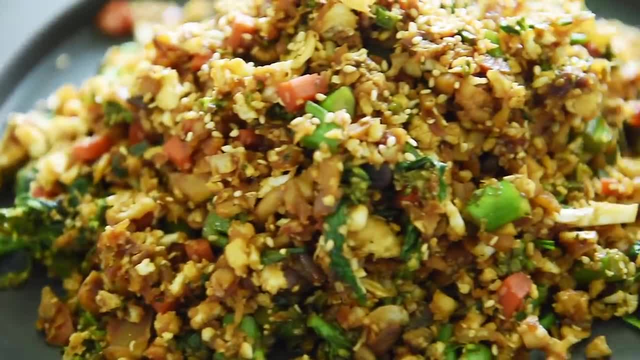 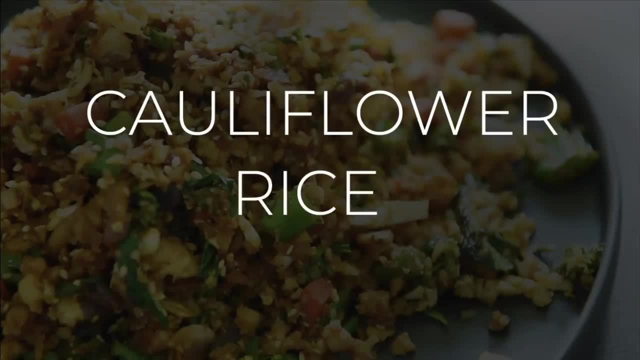 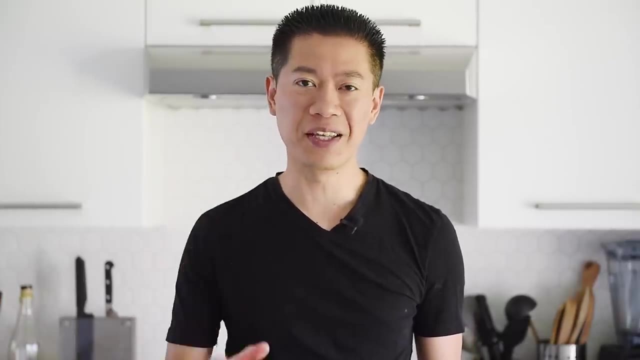 On today's menu. an easy recipe to put together. that's a bouquet of flavors. Delicious cauliflower rice, Le Homa. I'm Will Young from youngmancookingcom. Welcome to the channel where you can cook with confidence. I absolutely love fried rice and it's by far one of my favorite dishes of all time. 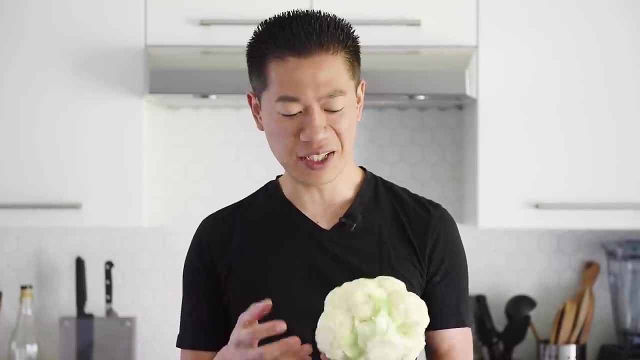 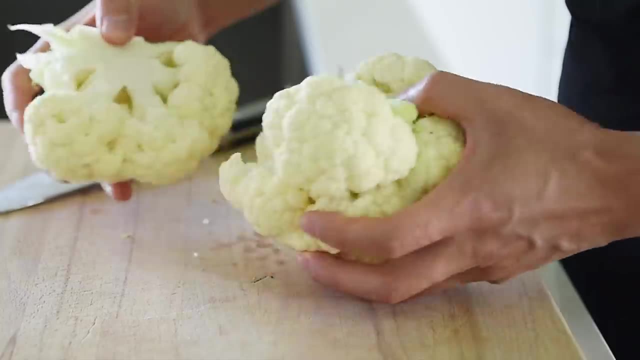 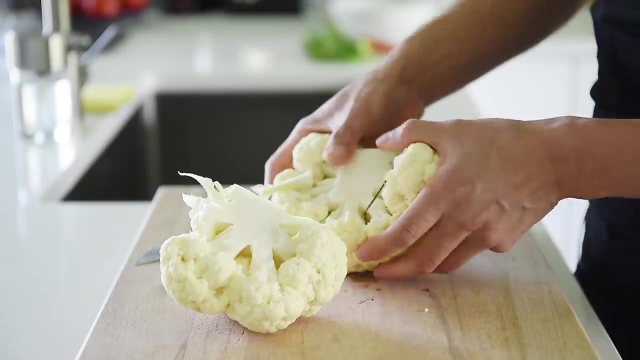 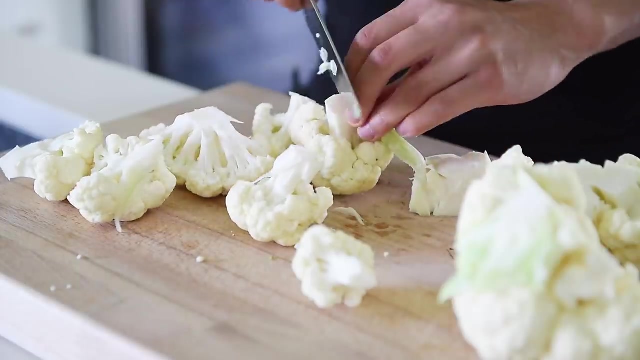 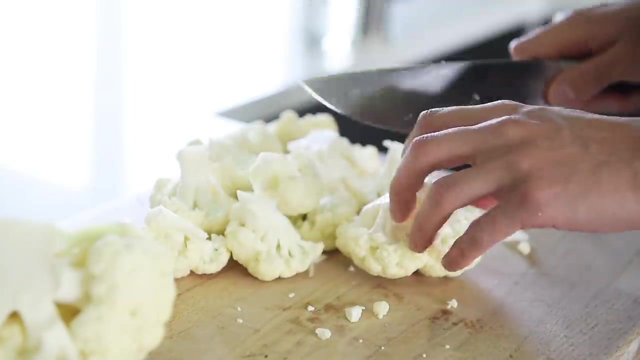 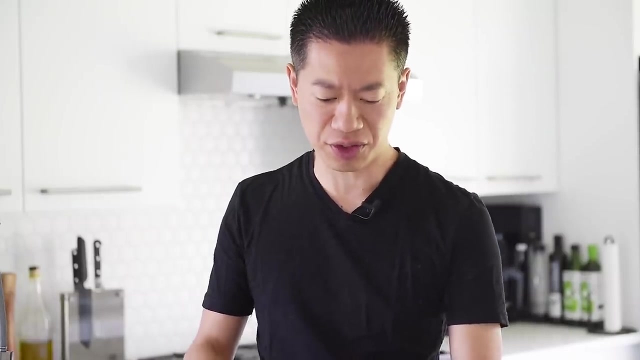 But if you don't have any rice on hand, that's totally okay. All you need is some amazing cauliflower. Prep one head of cauliflower by slicing into the stem and pulling out the florets. Chop the cauliflower down into bite-sized pieces. I find when you're prepping cauliflower or broccoli it's always best to kind of cut. 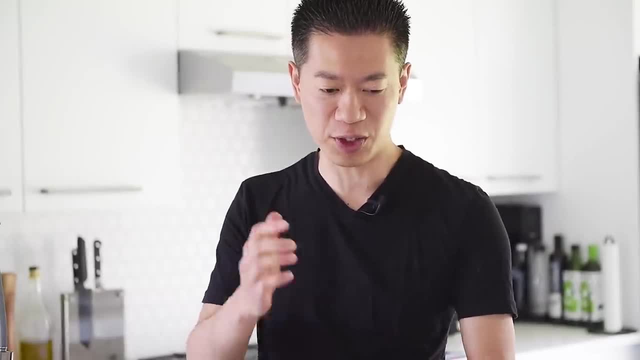 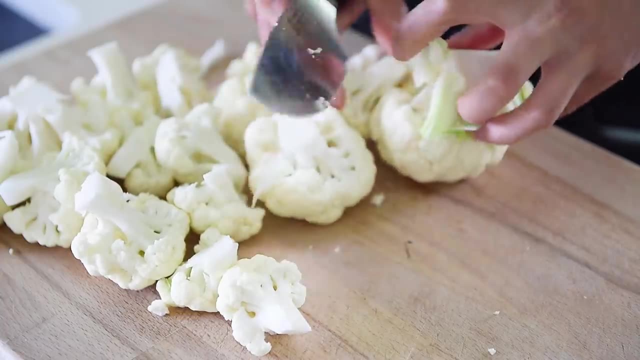 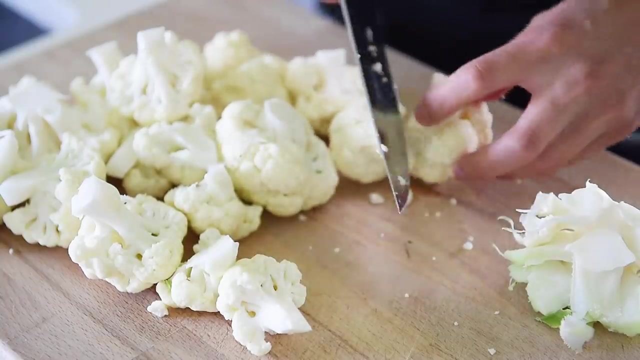 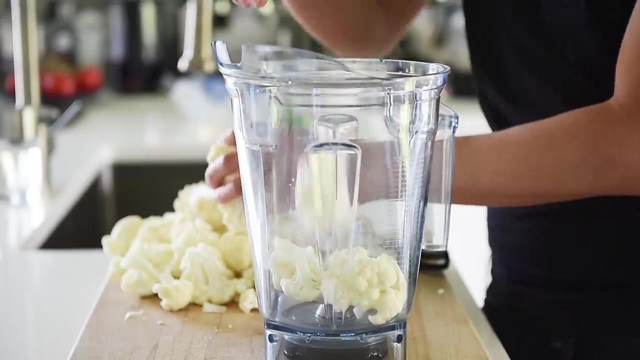 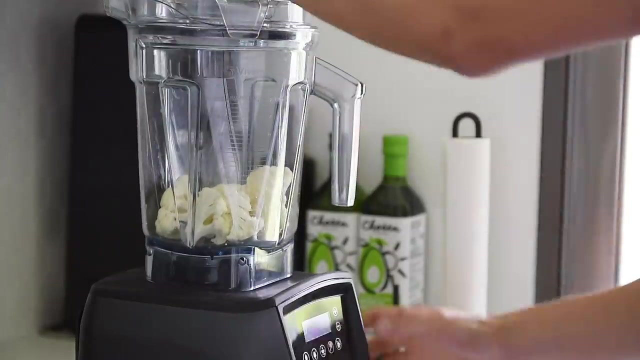 into the stalk and pull it apart rather than chopping the entire thing. This will give you a much cleaner cutting board Blender. Add some cauliflower to the blender. You'll need to rice the cauliflower a little bit at a time. Blend the cauliflower on the lowest setting for about 10 seconds. 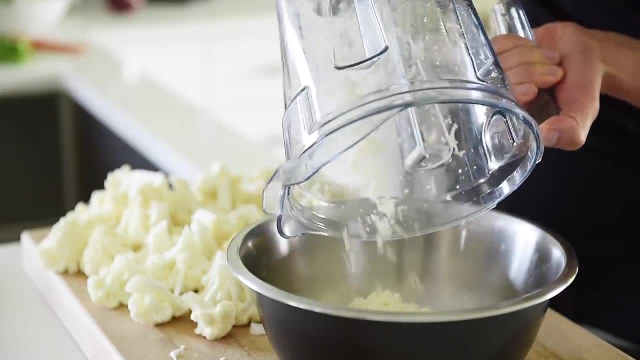 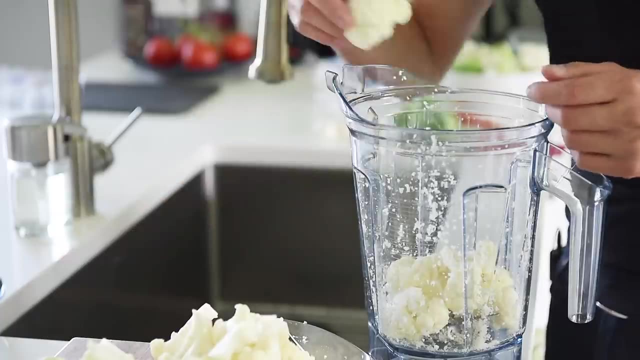 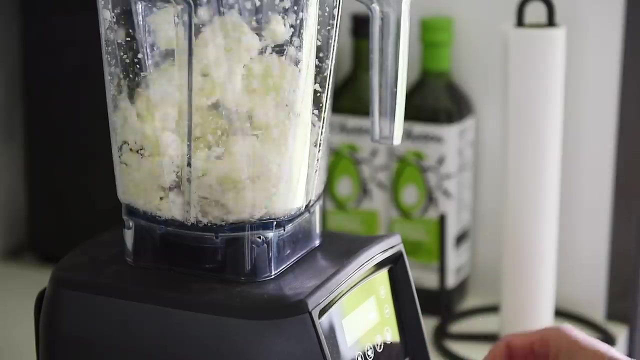 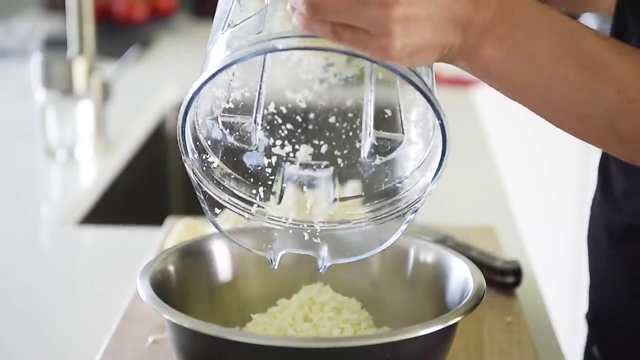 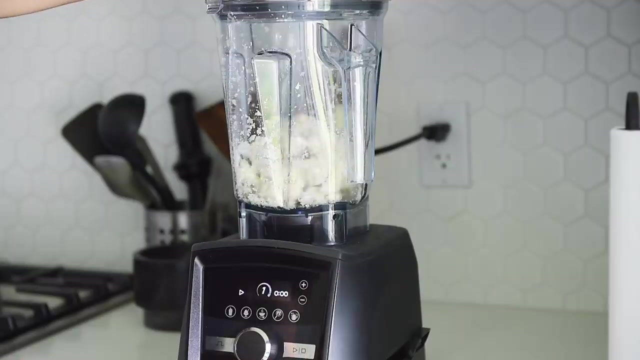 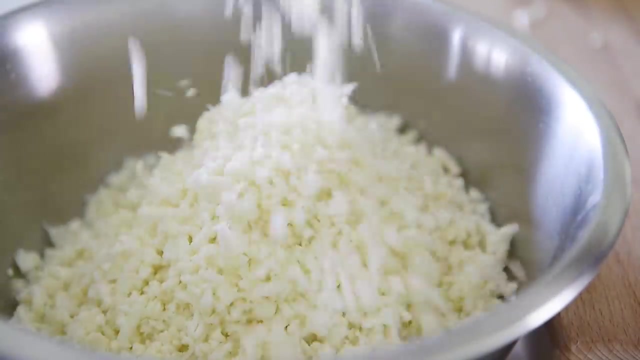 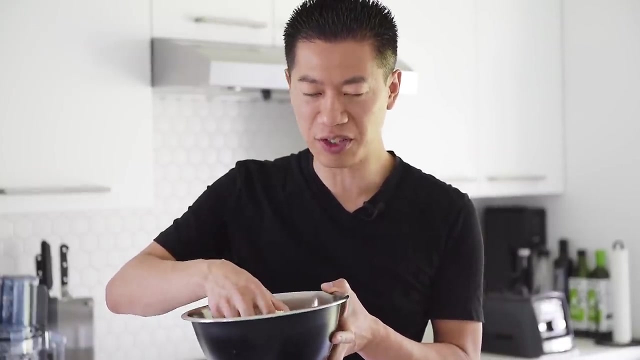 Pour out the rice cauliflower and repeat with the remaining florets. What I would recommend: mix. Consult my folio at the bottom of the blender. place the pumpkin in the blender and add some water. Takes a little bit of patience and, of course, you can buy frozen rice cauliflower. 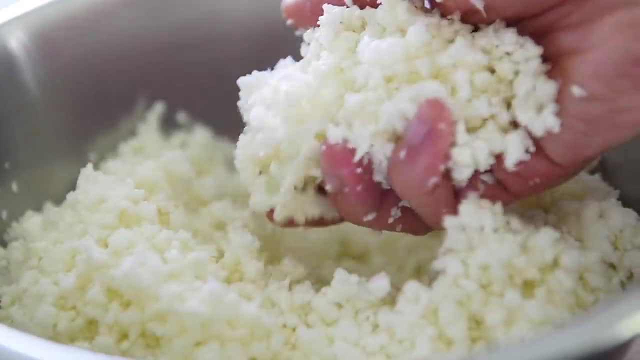 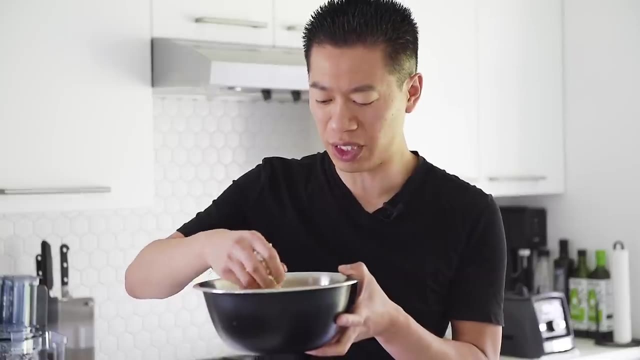 while you're at it, This one is also delicious with explicit ingredients. of course you can buy frozen rice cauliflower flour, but I find making it from scratch really gives it that incredible texture and keeps that al dente bite when you go and cook it. 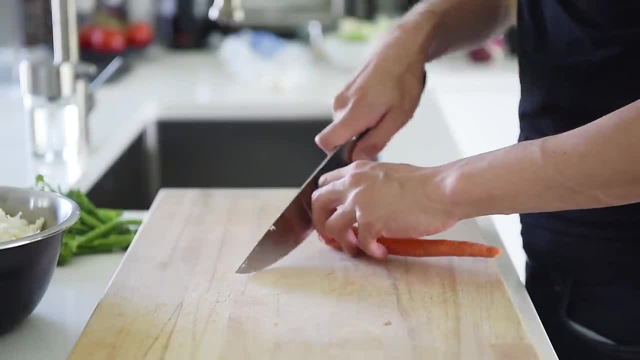 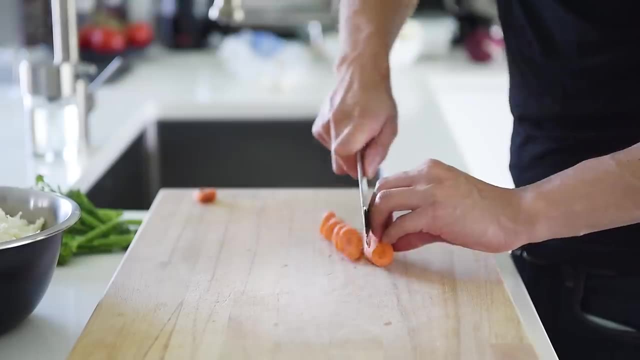 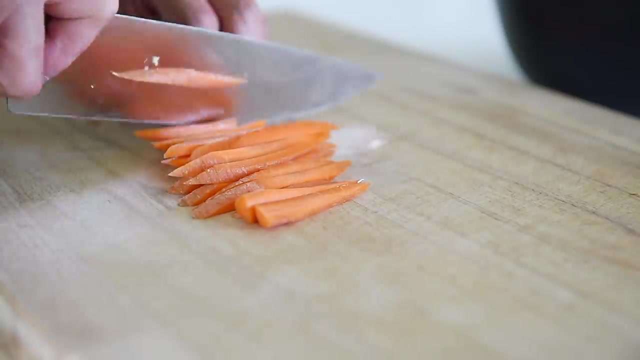 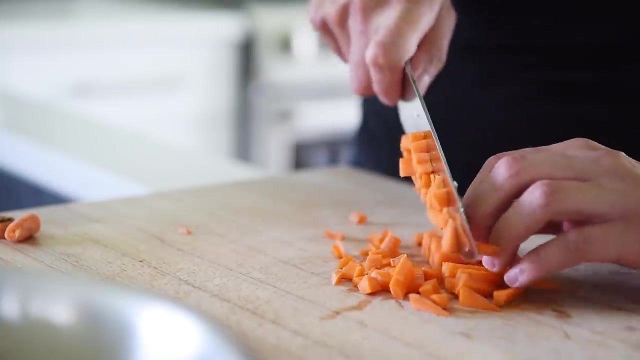 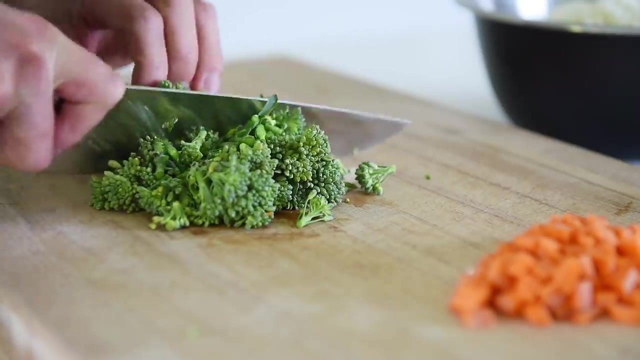 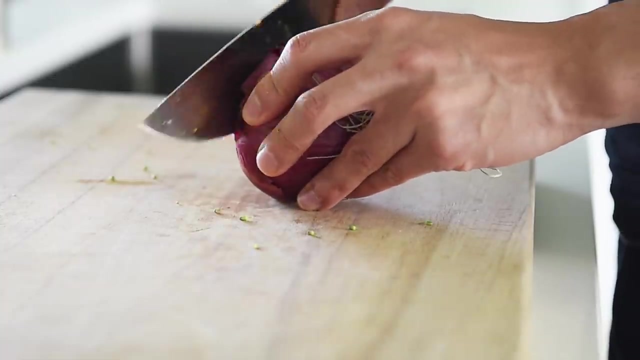 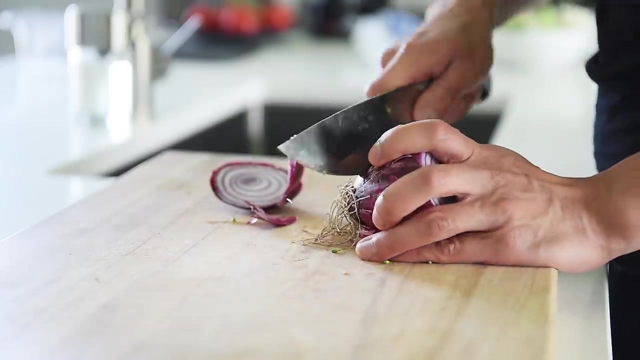 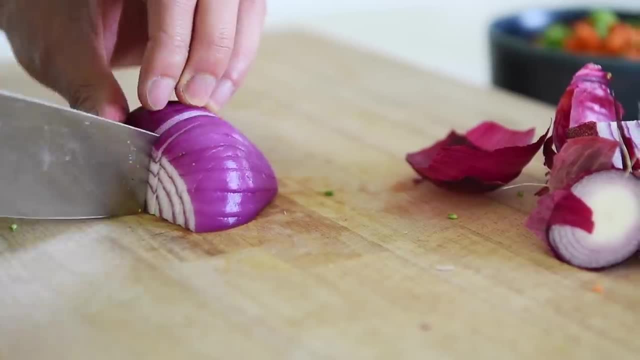 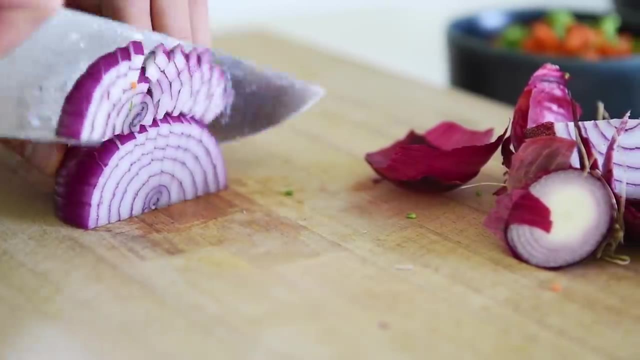 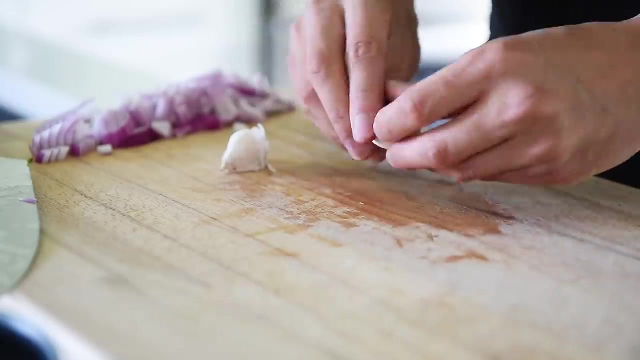 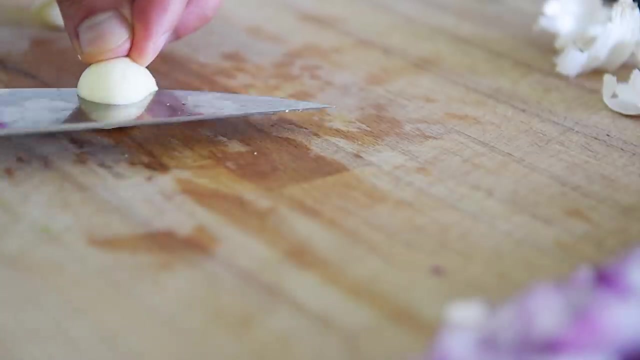 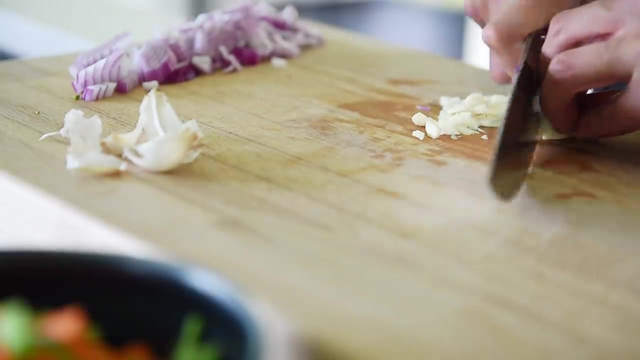 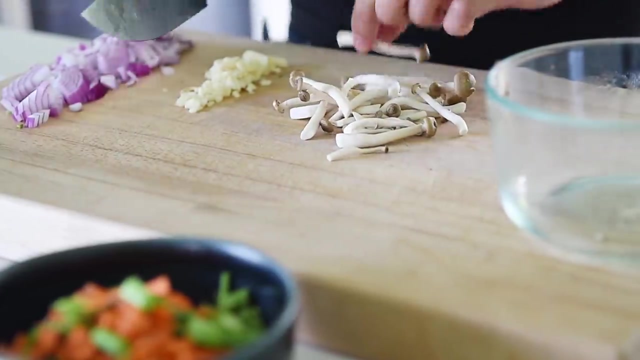 Half a red onion finely chopped. Half a red onion finely chopped. Two pieces of garlic finely chopped. About 30 grams of shimeji mushrooms chopped. About 30 grams of shimeji mushrooms chopped. About 30 grams of shimeji mushrooms chopped. 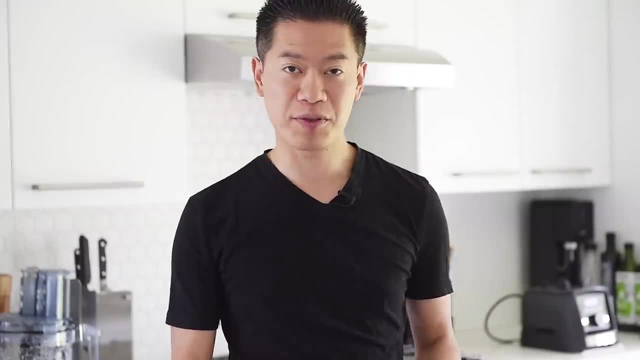 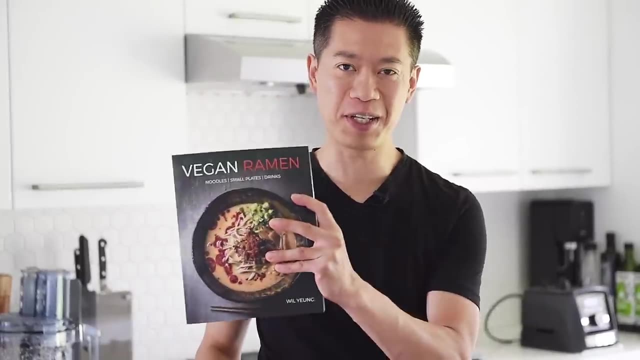 that's pretty much it. we just have to make a simple sauce and we're good to go super, super easy. and if you love easy recipes, like i do, of course, definitely check out that vegan ramen cookbook or the cook with confidence cookbook. i'll leave a link in the description box below. 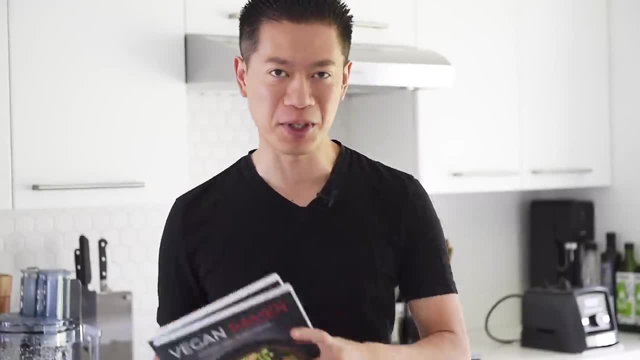 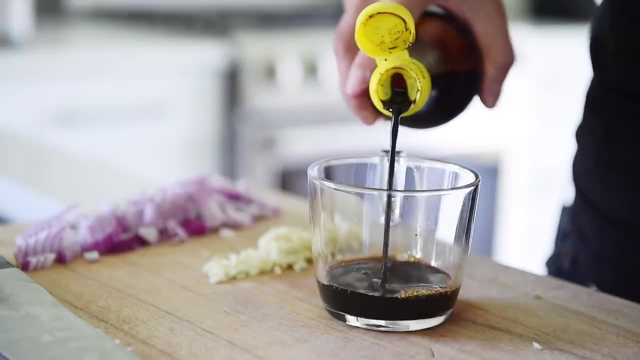 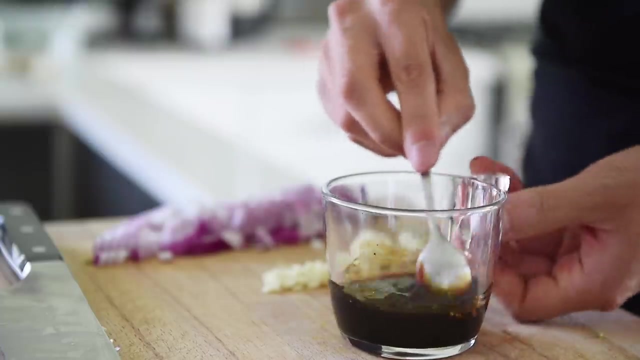 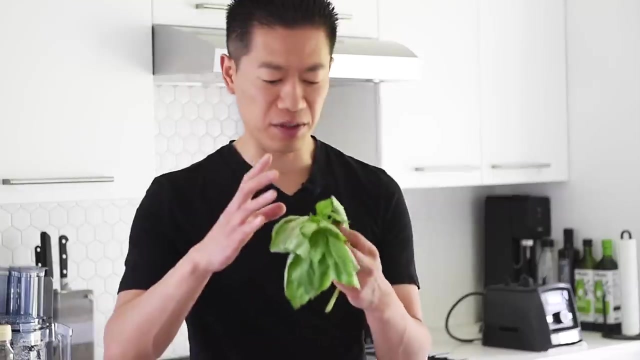 where you can check these out, get your signed copy or take a sneak peek inside the books. make the sauce by adding one tablespoon soy sauce, one teaspoon dark soy sauce, a splash of toasted sesame oil, one teaspoon hoisin sauce and stir. you also need some delicious, aromatic fresh basil- one of my favorite ingredients- and, of course, this. 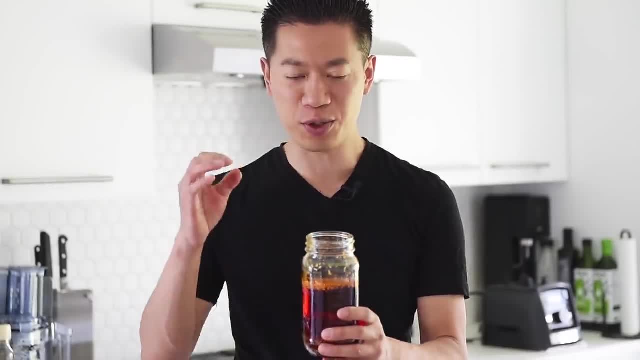 is not traditional in fried rice, but it's going to go incredibly well with the delicious smoky chili oil i made in the previous episode. you can make this really easily out of the oven and it's going to go incredibly well with the delicious smoky chili oil i made. 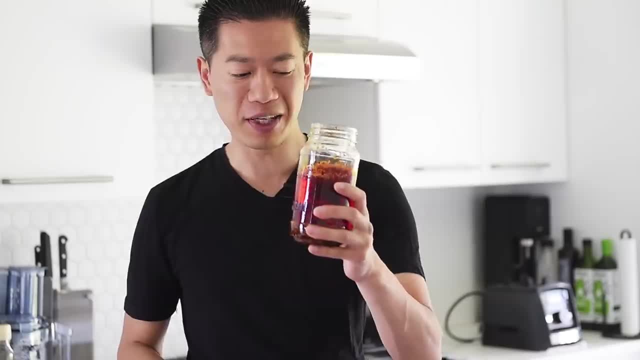 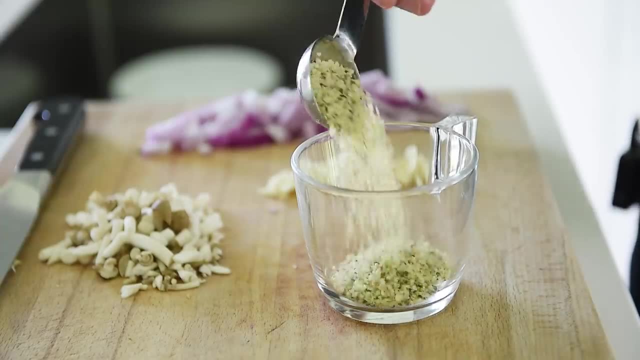 at home. i'll leave a link in the description box below where you can check this out, make this for yourself and see how amazing this is: two tablespoons hemp hearts, right. so this is not something i usually use on the show here, but it is something that i really. 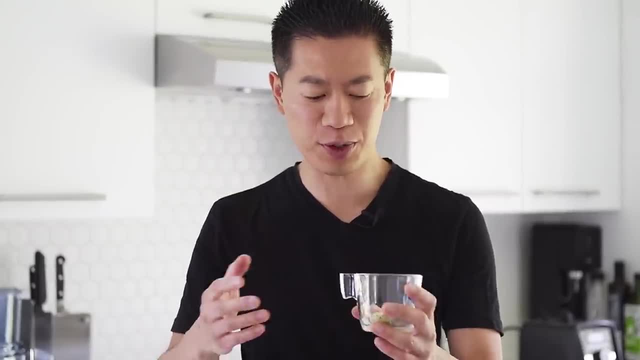 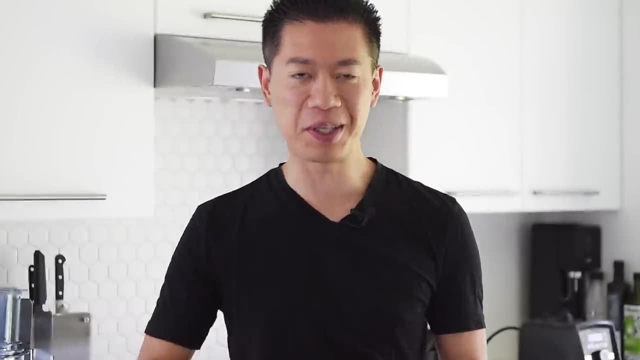 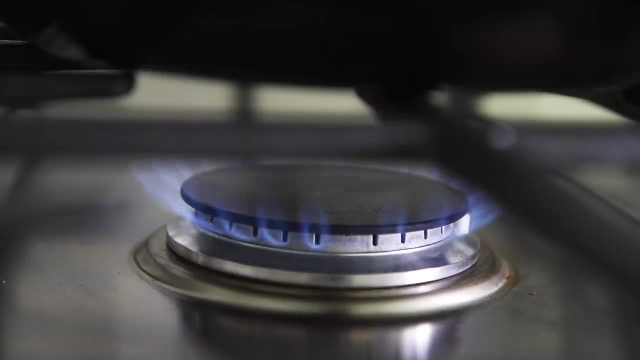 do enjoy. these are hemp hearts and definitely optional, but we'll add that a little bit of a crunchy salty earthiness to it. it's gonna be really nice and since we're in the spirit of being creative, why not? non-stick pan? medium heat. two tablespoons chili oil. 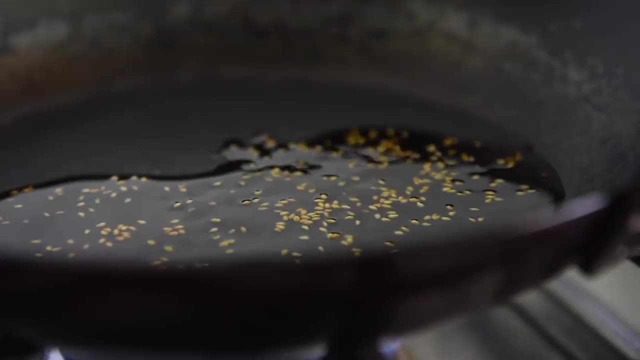 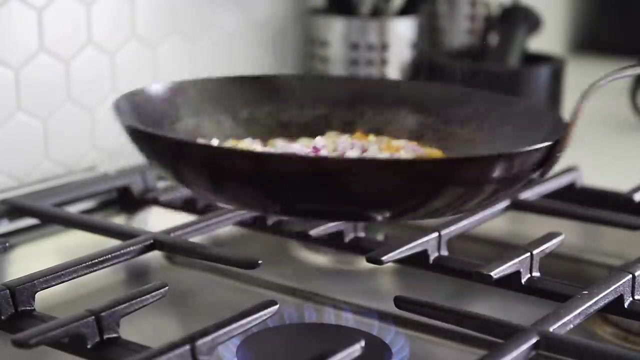 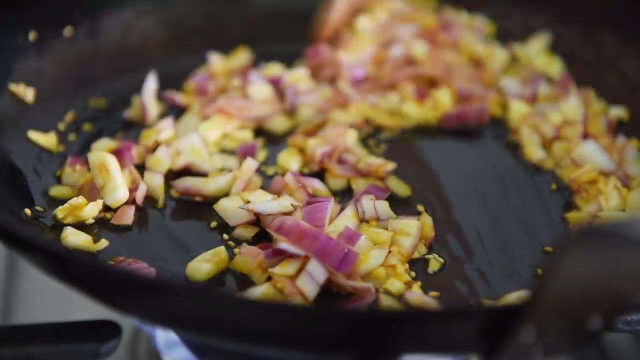 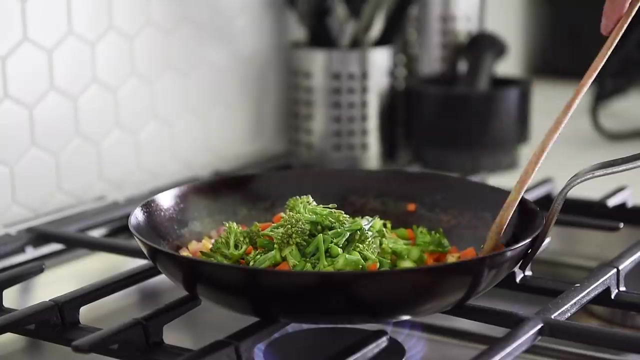 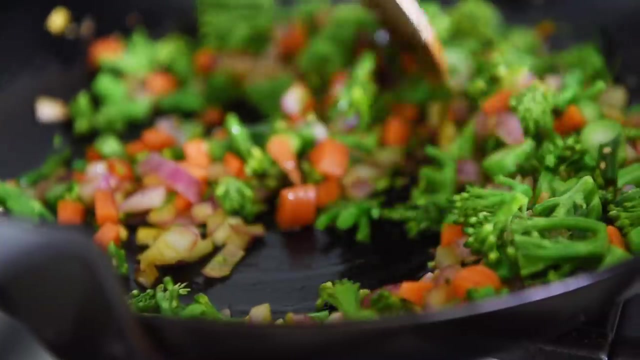 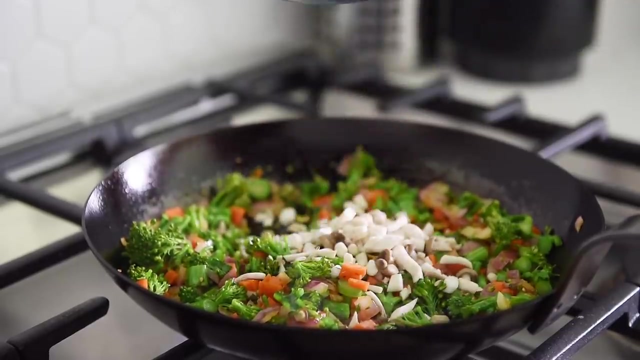 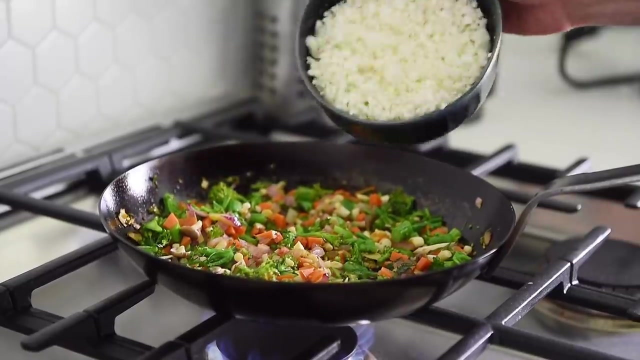 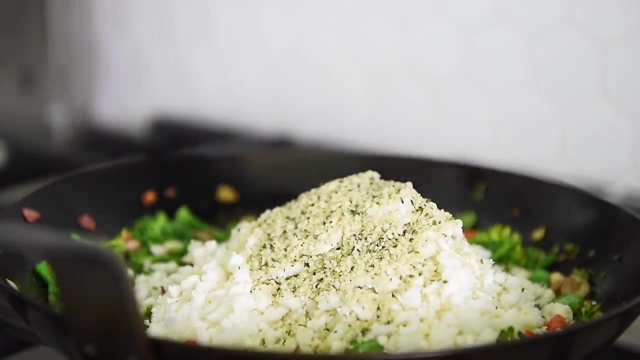 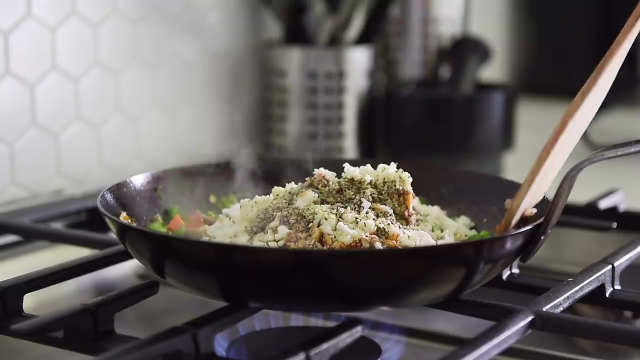 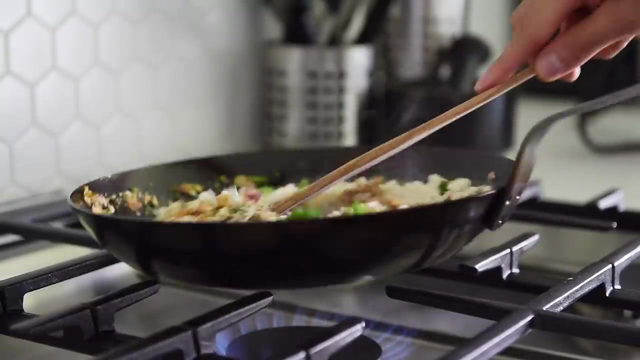 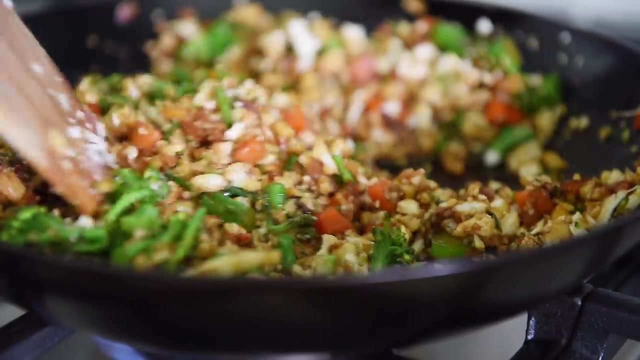 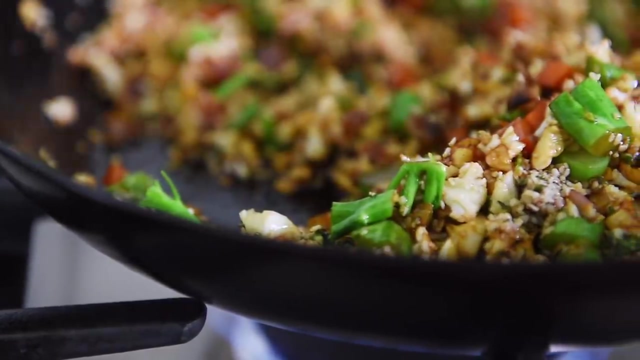 saute the onions and garlic for a couple of minutes. saute the carrots and broccolini for another couple of minutes. mushroom: two cups riced cauliflower, hemp hearts sauce. Temperature: stir-fry: 4 to 8 minutes. saute for three to four minutes. saute for three to four minutes. 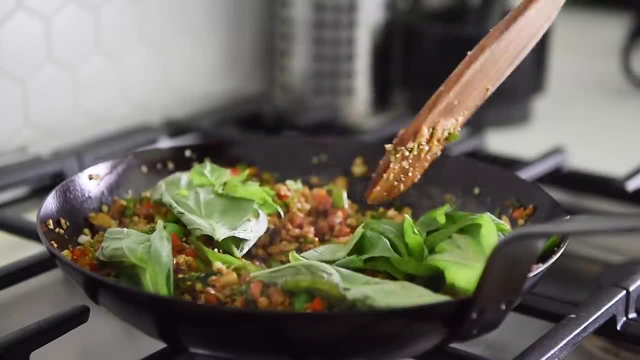 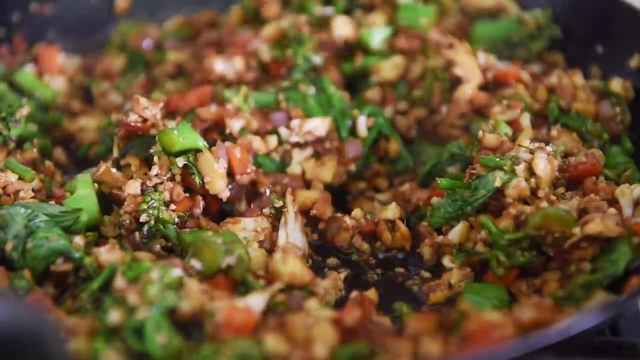 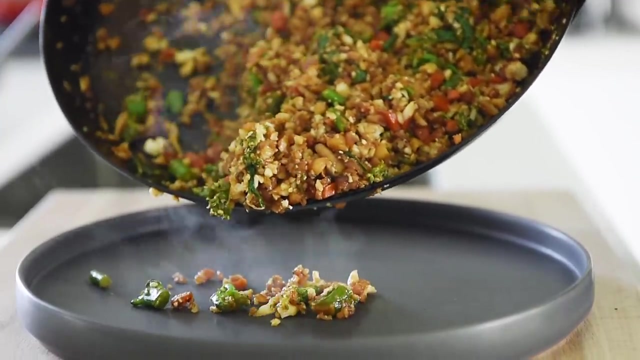 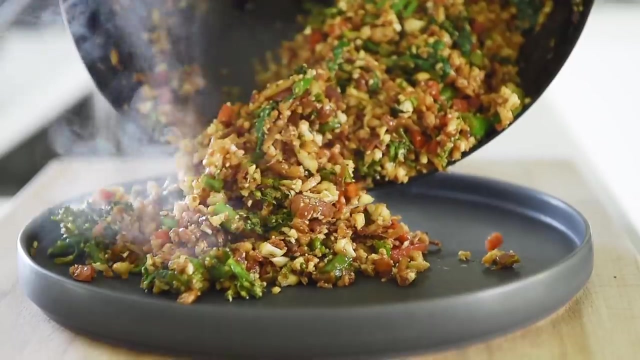 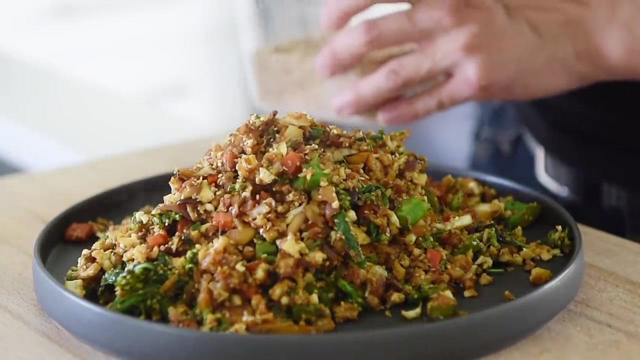 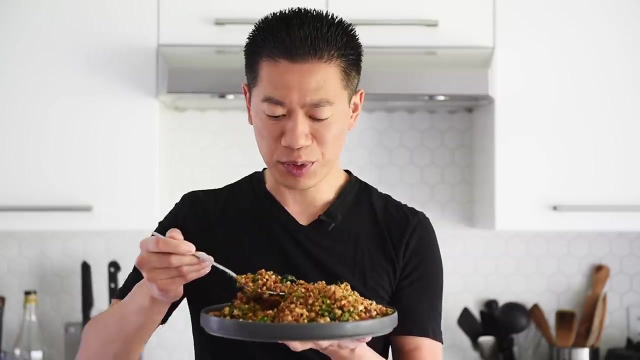 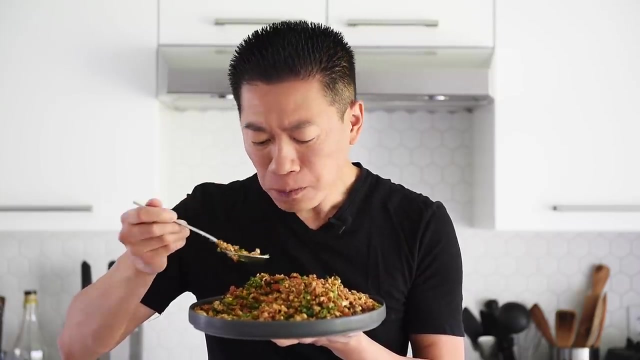 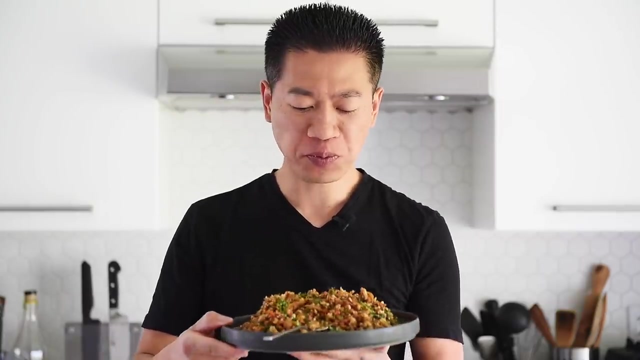 Kar, empty taste and give it a good stir. Plate, Top with sesame seeds and serve. You can now enjoy this delicious cauliflower rice with absolute confidence. It's simple, rustic dishes like this that gets me really excited about cooking food. Amazing, Just one bite and that is just full of flavor.